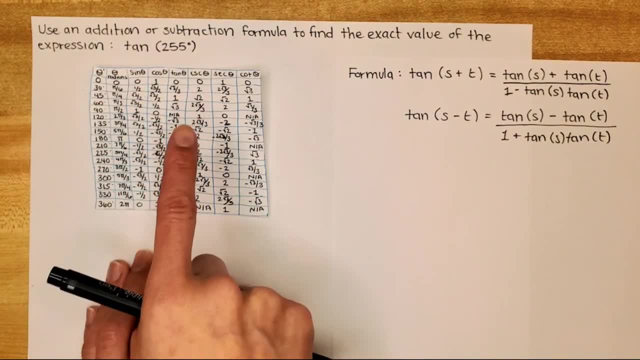 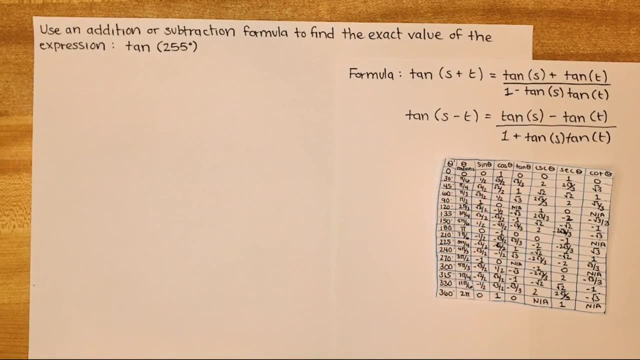 solve for that exact value of this particular expression, And so how we're going to do this is that we're going to go ahead and pick two values that equal 255 degrees. Whether it's subtracting it or adding it, it really doesn't matter, but as long as we picked two, 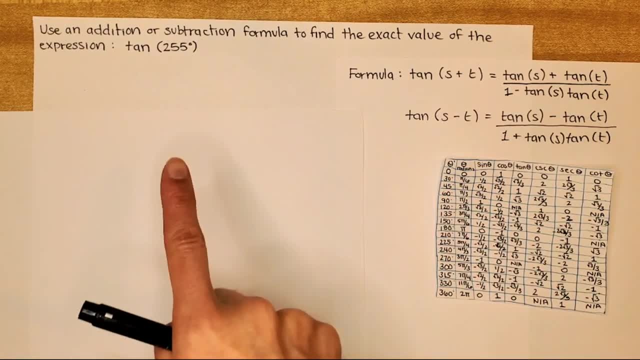 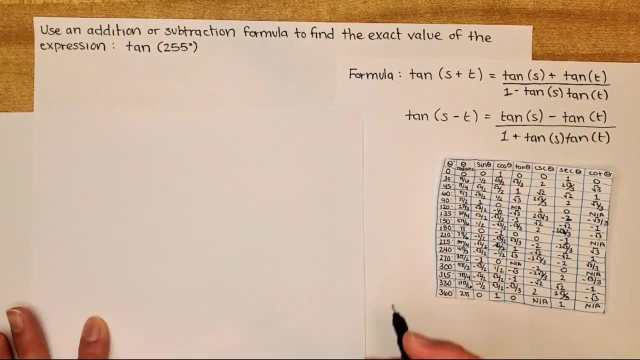 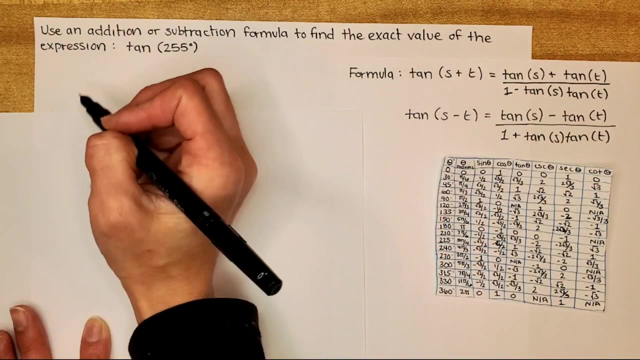 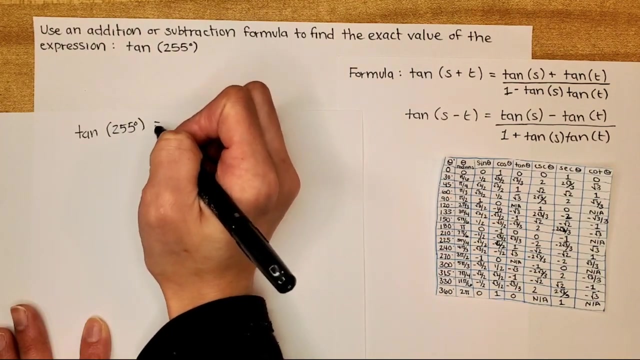 exact values given here in order to reach 255.. And so I'm going to use, for this example, the addition formula for tangent, and so we're going to do tangent of s adding with t, and so what that means is that we're going to take tangent of 255 and, like I said, we're going to find two angles. 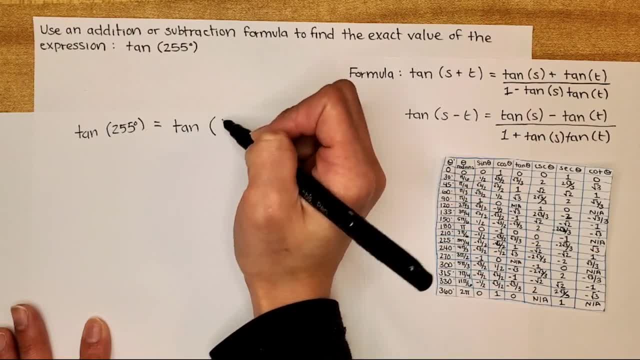 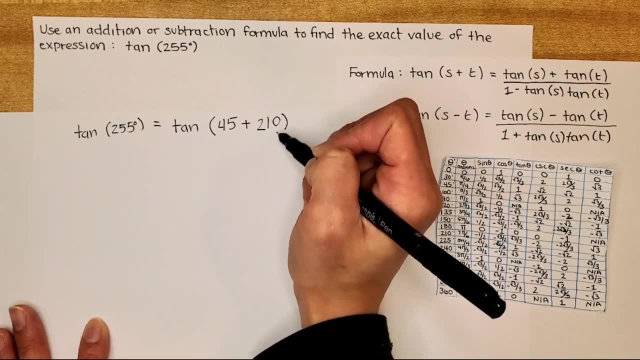 and so what I'm going to do is, using that addition formula is, find two angles, one of 45 and I'm going to use a special angle of 210, and so that will give me a total when you add 45 to 210, that's. 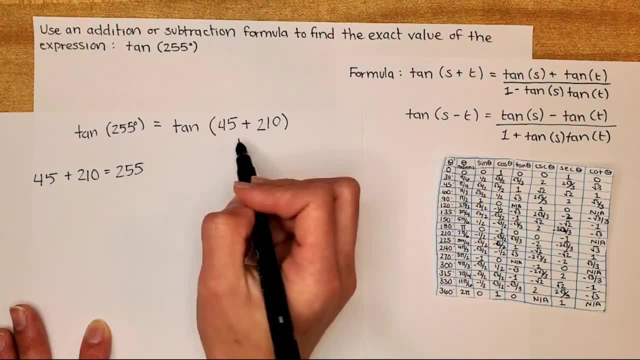 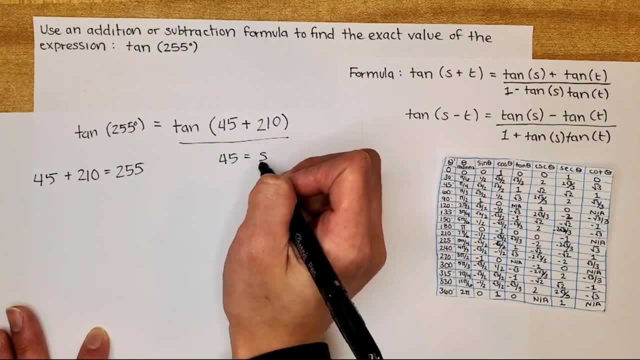 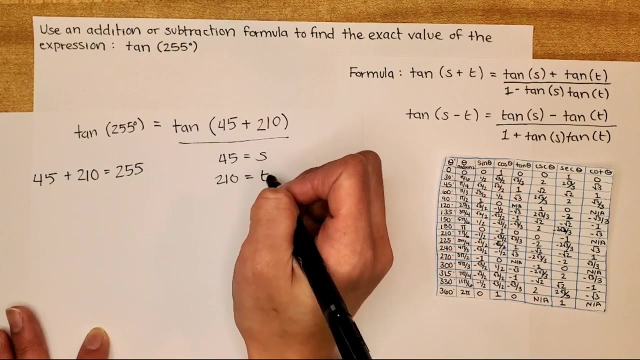 going to give you a total of 255, and so I'm going to use those values and plug them into the formula. my 45 is now equivalent to my s value in this formula, and my 210 value is equivalent to my t value, as you can see, and so when we plug that, 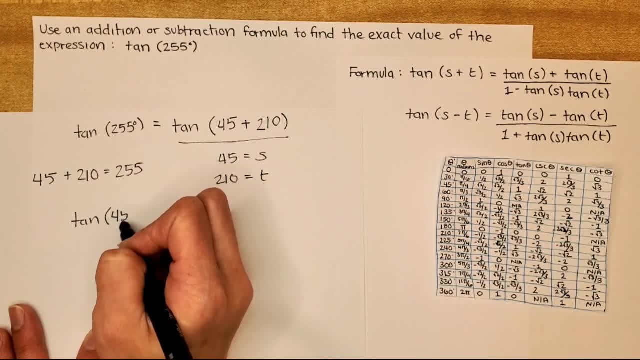 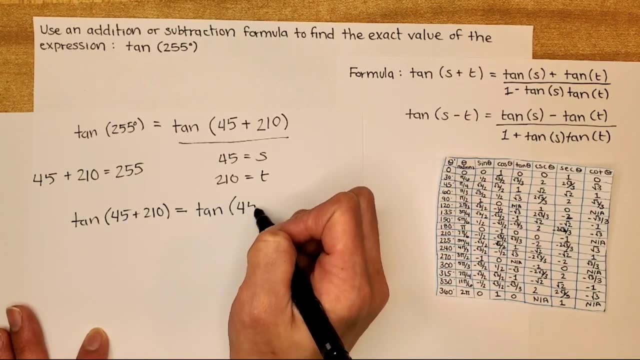 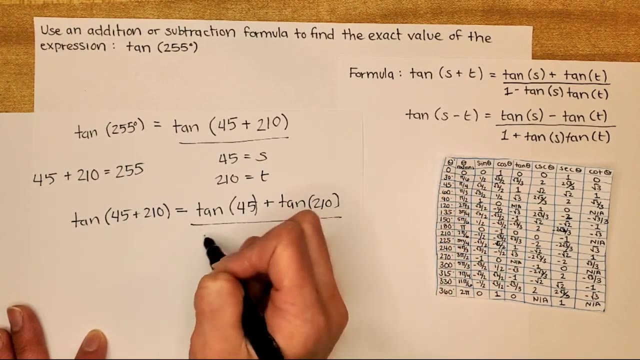 straight in. that's going to give you a total of 255, and so I'm going to use a special angle of 210 into that formula: Tangent of 45 plus 210 equaling tangent 45 plus tangent of 210 over one, minus tangent of 45. 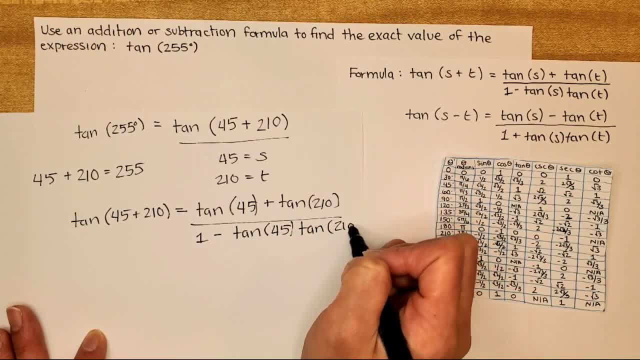 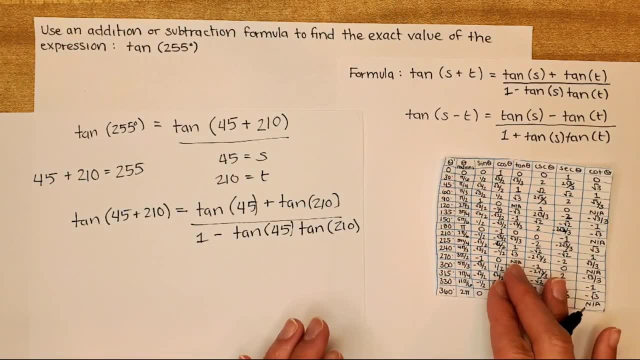 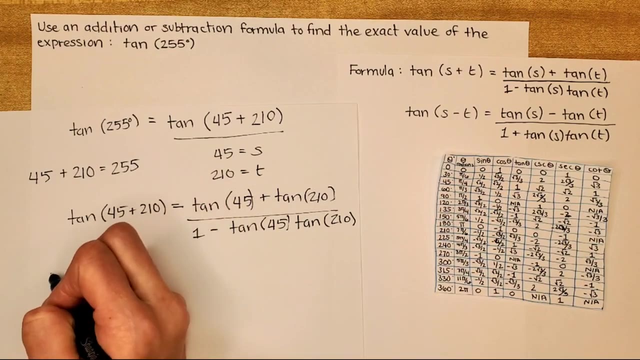 multiplied by tangent of 210.. We have to just essentially replace each of these values with an exact value of tangent to tangent of 45 and tangent of 210.. And so when we discover what the value of tangent 45 is, you can see right here is that we have the value of one. 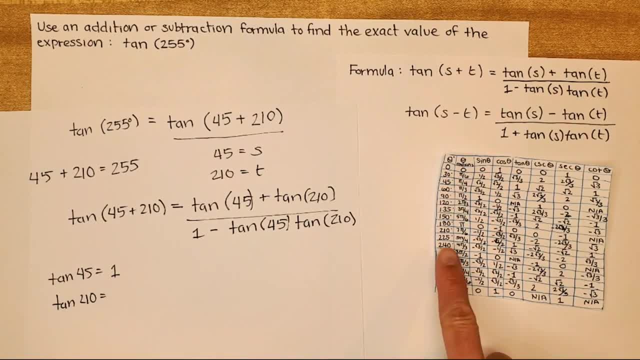 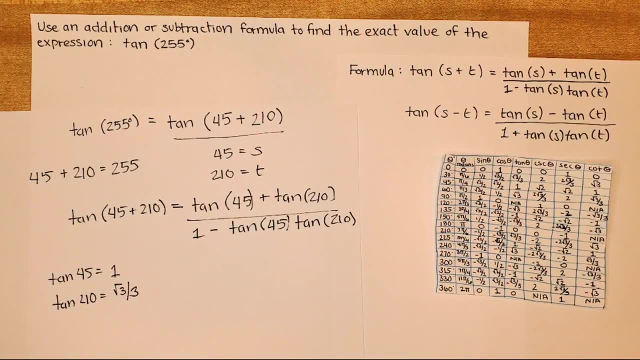 And tangent of 210 gives us the value of square root of three over three, And so what that essentially means is that we're going to replace each of these values into our formula to then find that exact value. So, tangent of 45, we determined that's going to be one. 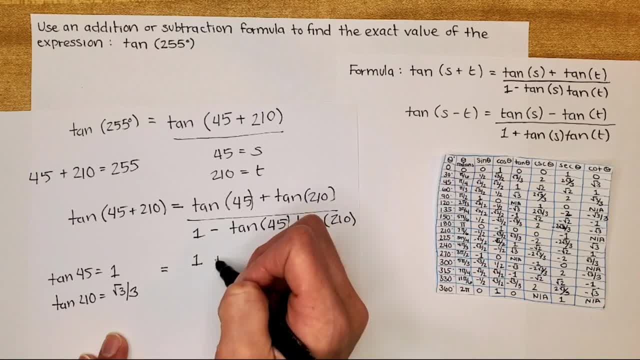 And then we also have the tangent of 210, which that puts us at a square root of three over three, And that puts us over one minus one times the square root of three over three. Now, what does that exactly mean in this case scenario? 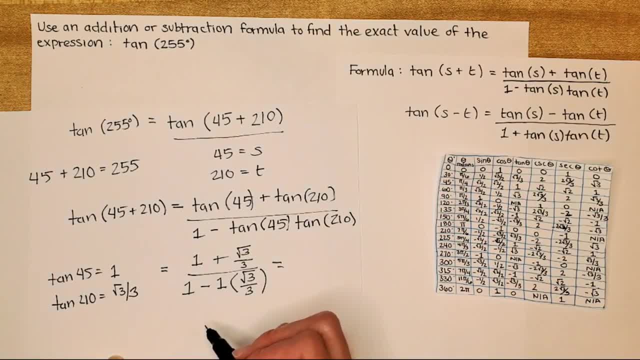 Well, now, what we're going to do is that we're just going to go ahead and simplify that, And so, once we simplify that down, we are gonna be given, all right, one plus square root of three over three, with one minus square root of three over three. 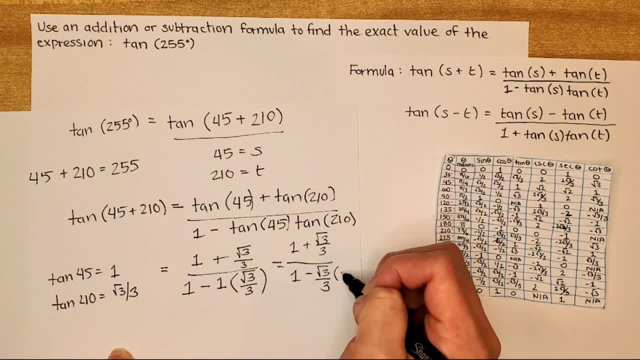 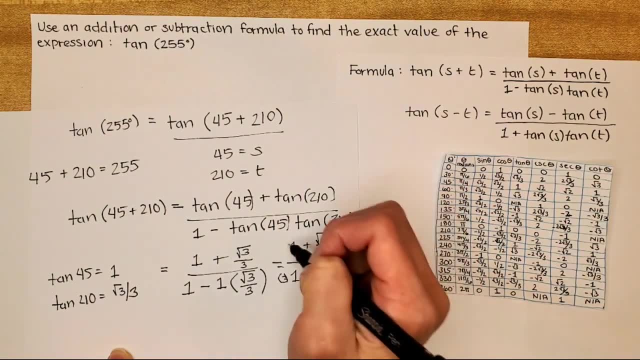 And so that's going to give us. we've got to find our common denominator here. Okay, let's multiply all those sides by 3.. All right, and that's going to give us a total of 3 plus the square root of 3 over 3, minus the square root of 3.. 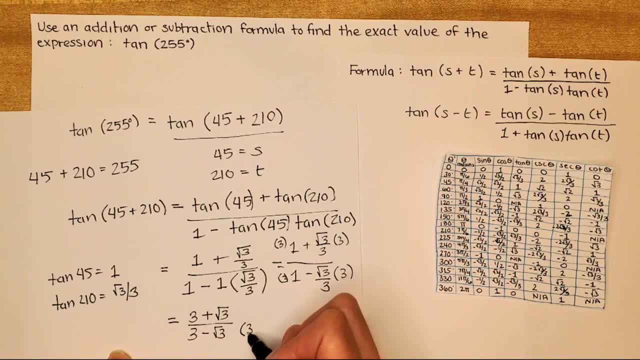 Now we're going to go ahead and take the reciprocal value in order to get rid of that square root value right there at the bottom, And so when we do that, we're going to then be left with 9 plus 6, the square root of 3, plus 3 over 9 minus 3.. 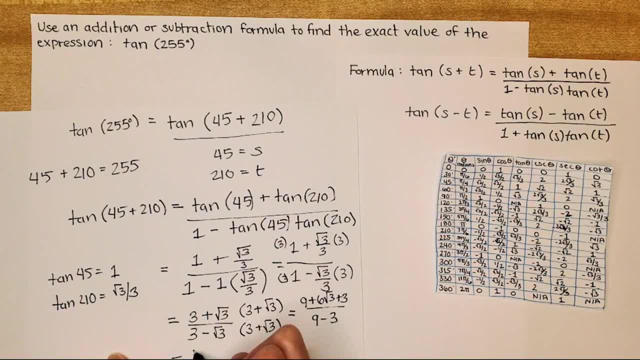 And so, as you can see, when we continue to reduce it down, we'll get 12 plus 6 square root, The square root of 3 over 6.. And we can continue to even simplify that by the common denominator of 6..